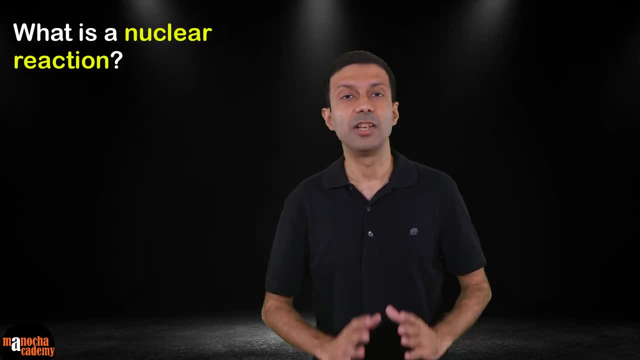 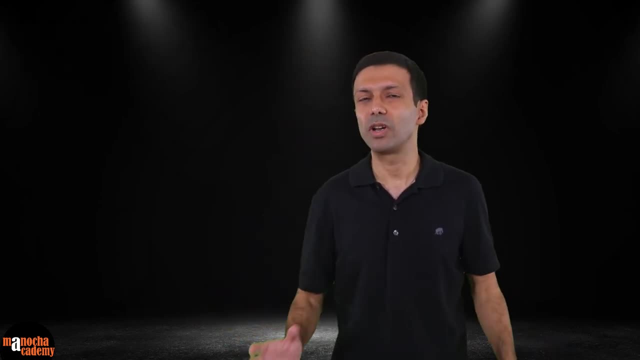 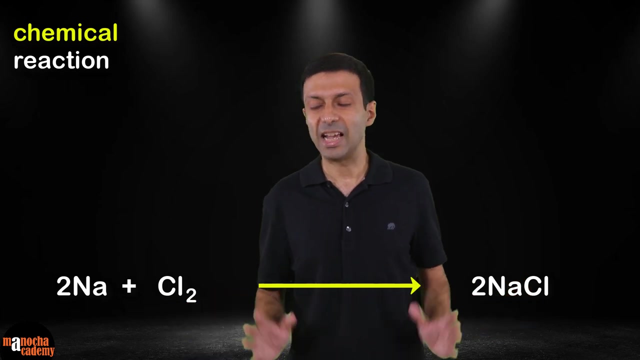 reaction. Yes, chemical and nuclear reactions are very different. Let's compare them. I am sure you have seen that the chemistry textbook is full of chemical reactions. Here is a simple example of a chemical reaction. As you can see, sodium reacts with chlorine to form the compound sodium chloride. In this 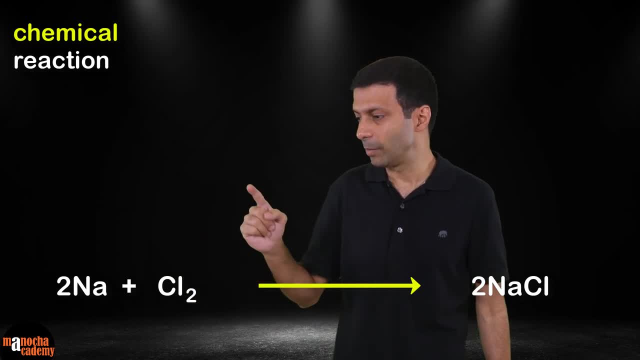 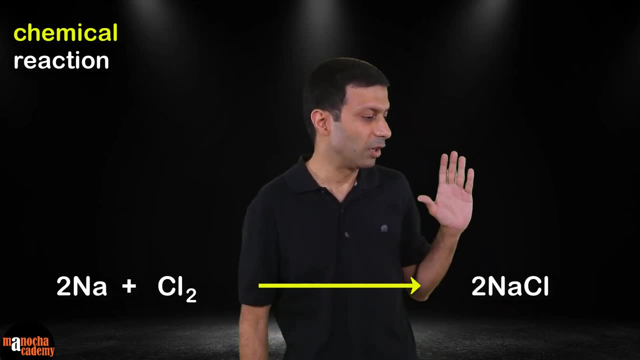 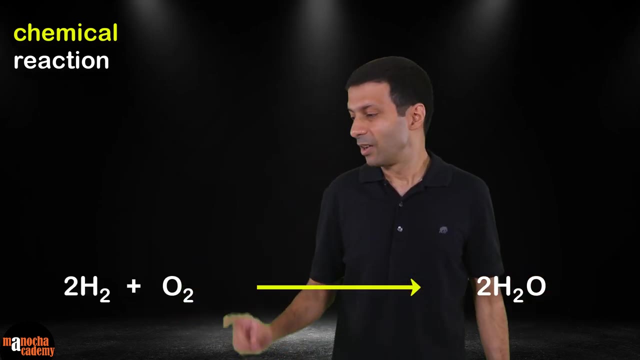 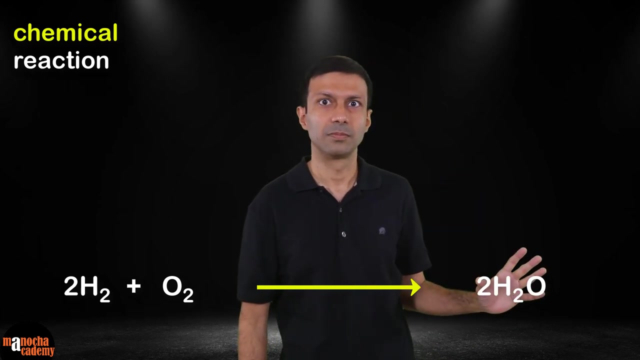 reaction an electron is transferred from the sodium atom to the chlorine atom, And so an ionic bond is formed And this forms the compound sodium chloride. Here is another simple example of a chemical reaction. Here the hydrogen and oxygen atoms share electrons to form the compound water. So chemical reactions involve the transfer or sharing of electrons. 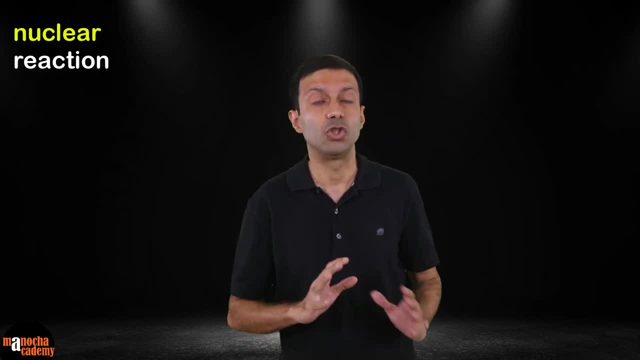 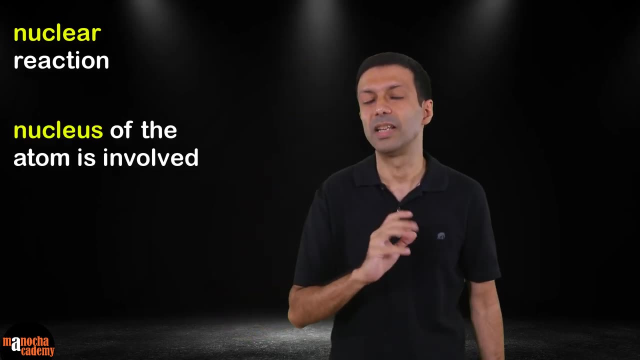 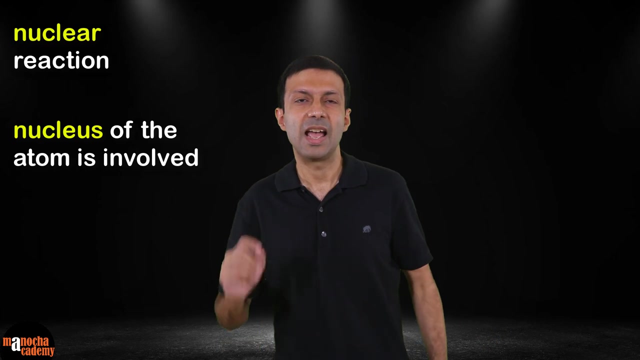 But nuclear reactions are very different. They don't involve the electrons of the atom. In nuclear reactions, the nucleus of the atom is involved. The nucleus changes And that's why they are called nuclear reactions. As you may know, that the nucleus of an atom contains 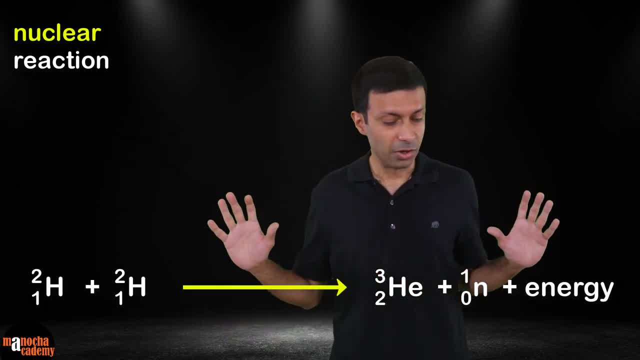 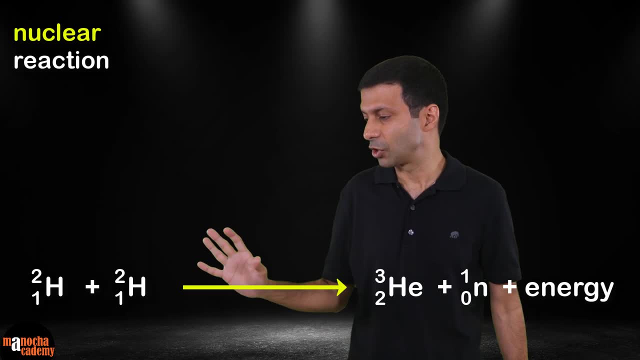 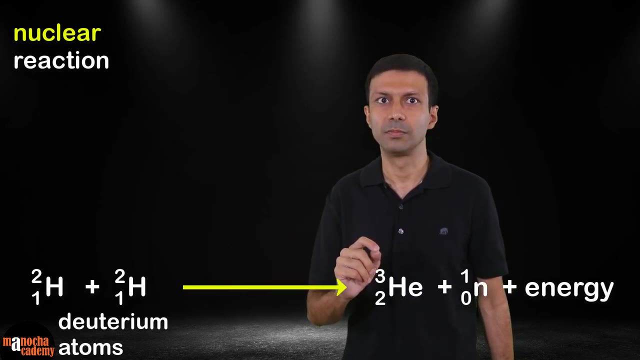 electrons, And so here is an example of a nuclear reaction for you. Now, one interesting thing that you can see here: in this nuclear reaction, on the left side there is deuterium atoms. These are isotopes of hydrogen, But there is no deuterium. 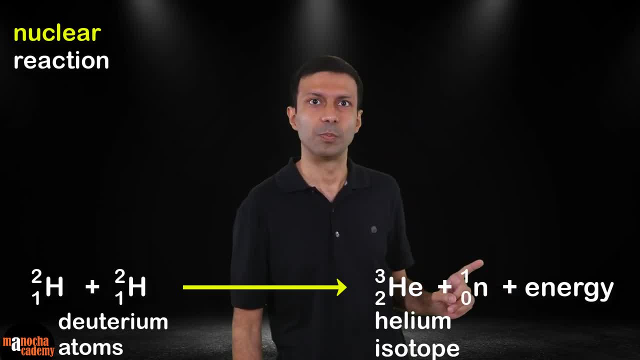 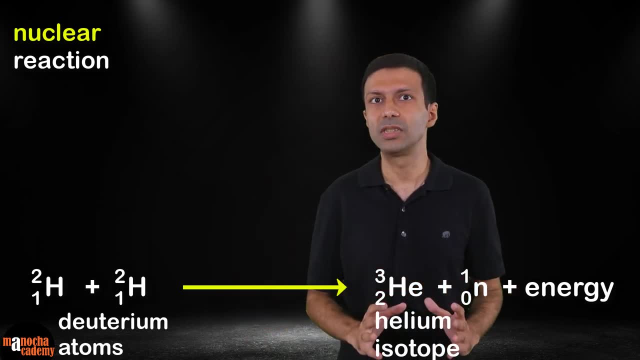 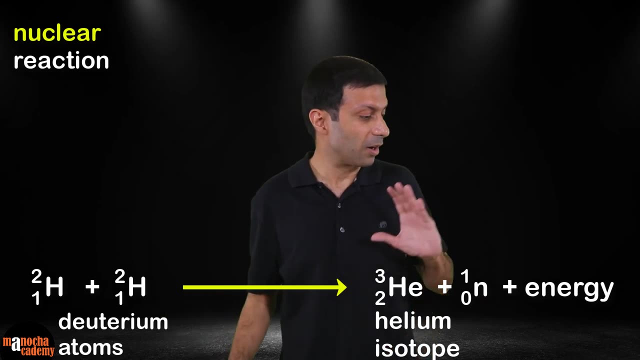 on the right side There is a helium isotope. The atom has changed completely. Now why is that? Why? Because the nuclear reactions involve the change of the nucleus, And when the nucleus changes, then the atom changes into a completely different atom. 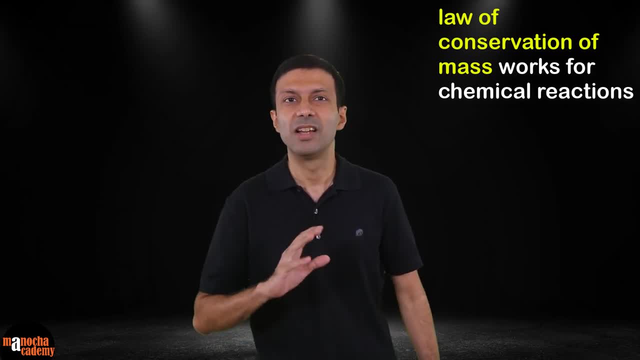 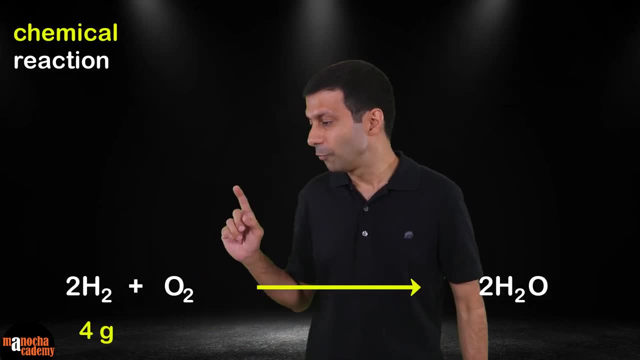 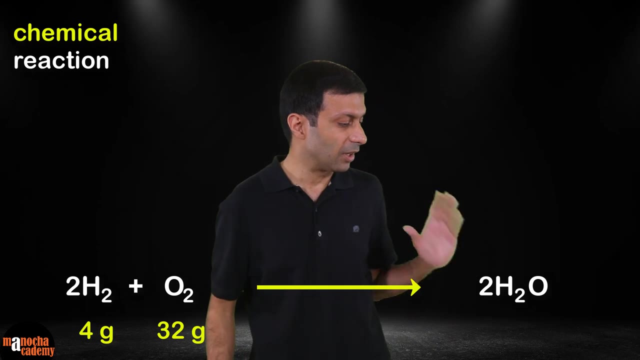 Another important difference is that the law of conservation of mass works for chemical reactions but not for nuclear reactions. For example, if you take 4 grams of hydrogen gas and you combine it with 32 grams of oxygen gas, then you are going to get 36 grams of. 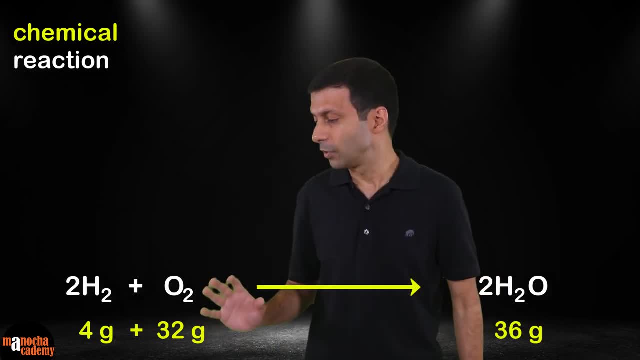 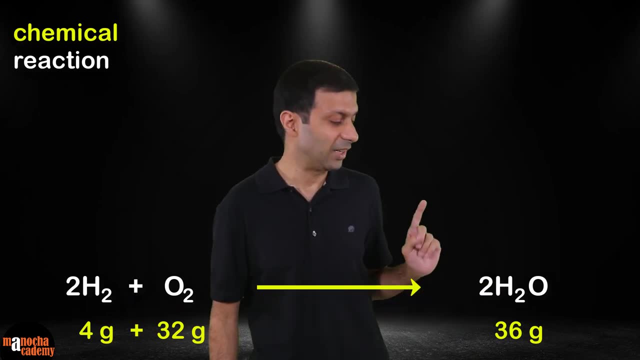 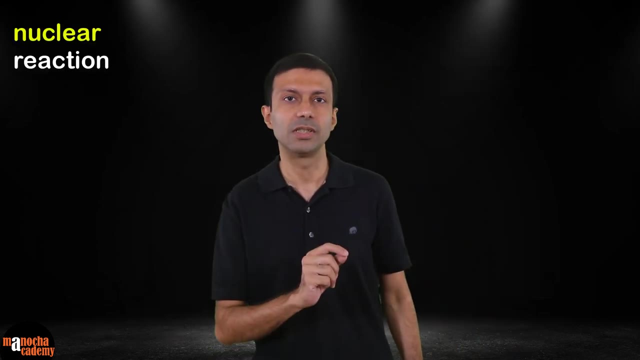 water. As you can see, the total mass of the reactants is 36 grams And it's exactly equal to the total mass of the products- 36 grams. So the law of conservation of mass is satisfied here. But in nuclear reactions the law of conservation of mass is not satisfied. Let's take some. 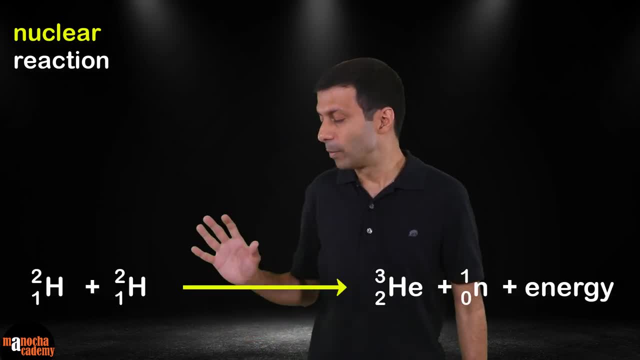 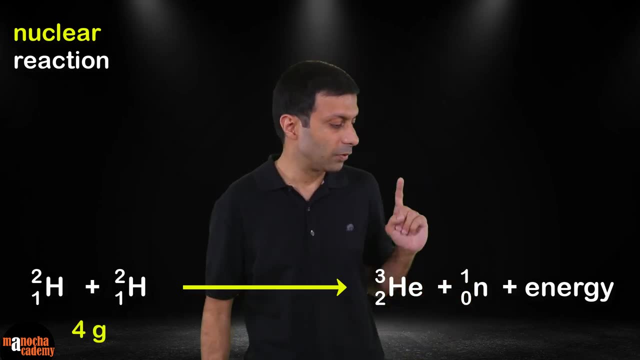 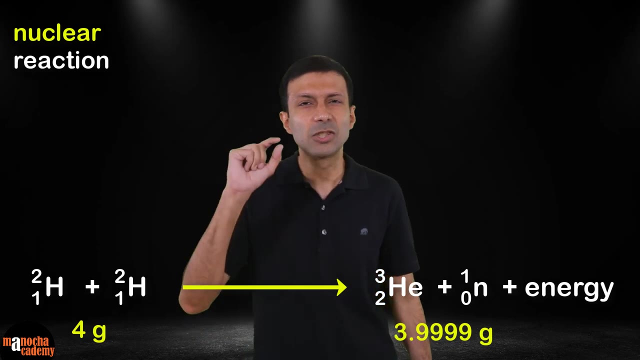 numbers as an example. So let's say, the total mass of the reactants here, which is the isotopes of hydrogen, is 4 grams, But the total mass of the products is 3.9999 grams. So can you see that there is a small 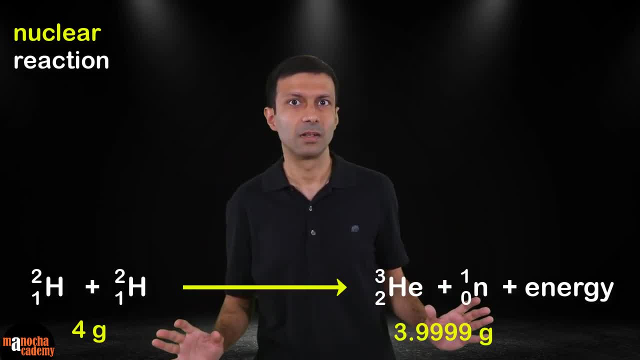 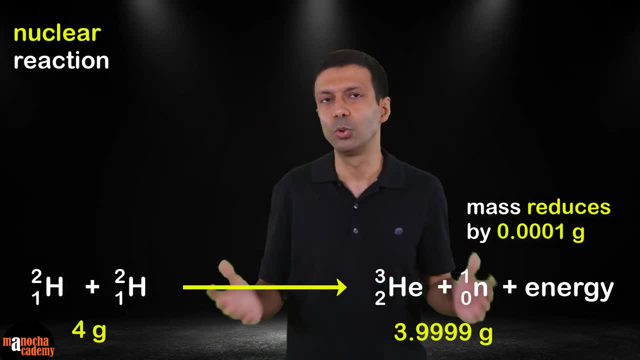 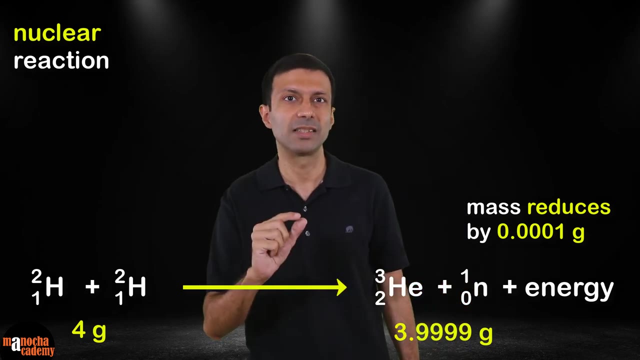 loss in mass. in this nuclear reaction, The mass reduces by 0.0001 grams. Now what happens to this mass? Is it a measurement error? No, There is actually a small loss in mass and it gets converted into energy, In fact a lot. 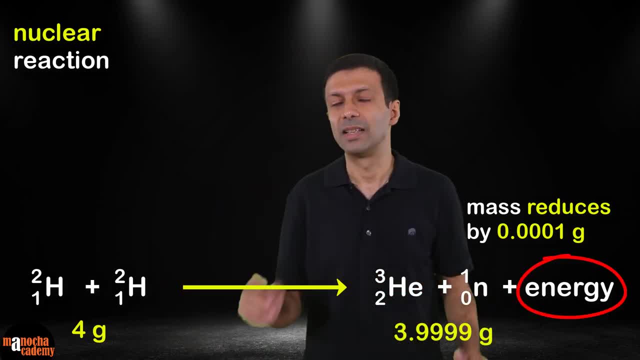 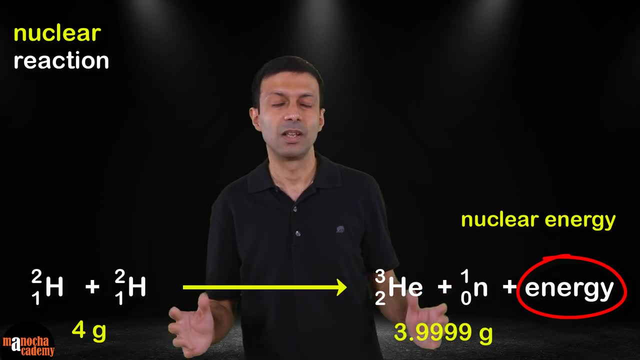 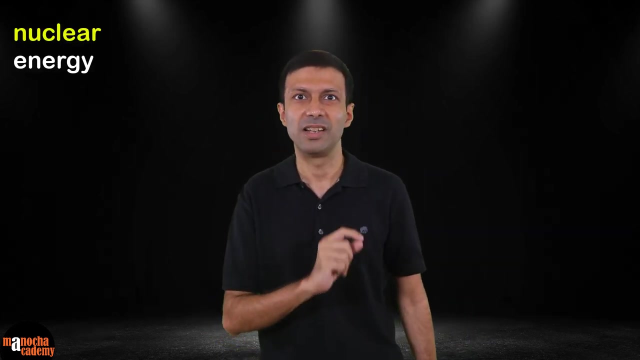 This is nuclear energy, the energy released during a nuclear reaction. The nuclear energy is usually released in the form of heat and light energy. Now how much energy is released? We can calculate the amount of energy produced using Einstein's famous equation: E equal to mc2,, where m is the loss in mass. 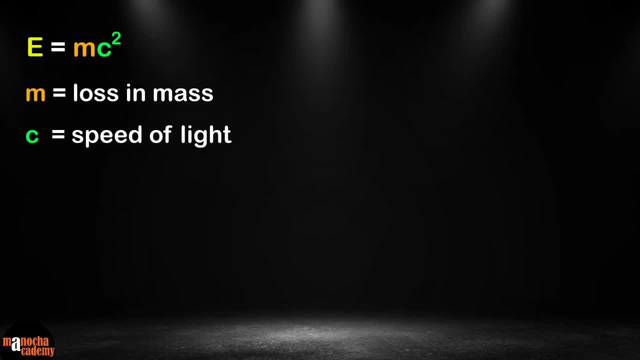 So we can calculate the amount of energy produced using Einstein's famous equation: E equal to mc2, where m is the loss in mass, C is the speed of light. If in a nuclear reaction the loss in mass is 0.0001 gram, then let's calculate how much. 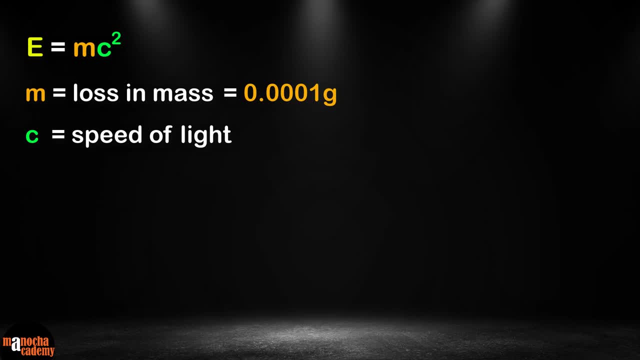 energy is produced. First let's convert the mass into SI unit, that is kgs, And now let's plug in the speed of light, which is 3 into 10 to the power, 8 meter per second square. So the amount of energy works out to be 9 into 10 to the power, 9 J. 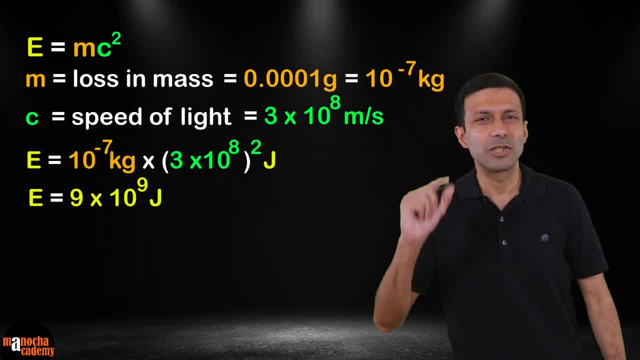 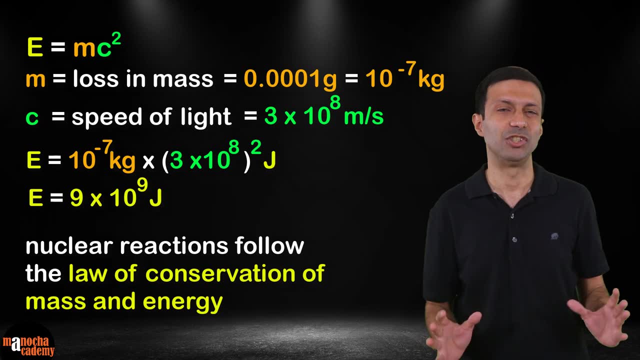 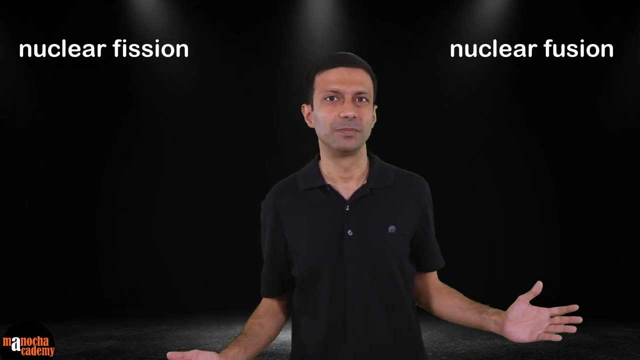 That's a lot of energy for a small loss in mass. So nuclear reactions follow the law of conservation of mass and energy. There are two types of nuclear reactions: nuclear fission and nuclear fusion. We will discuss both fission and fusion and then compare them. 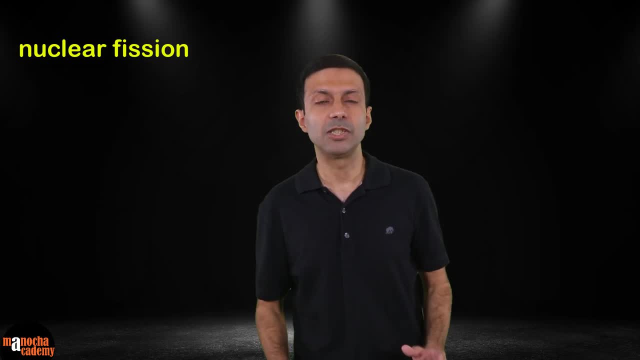 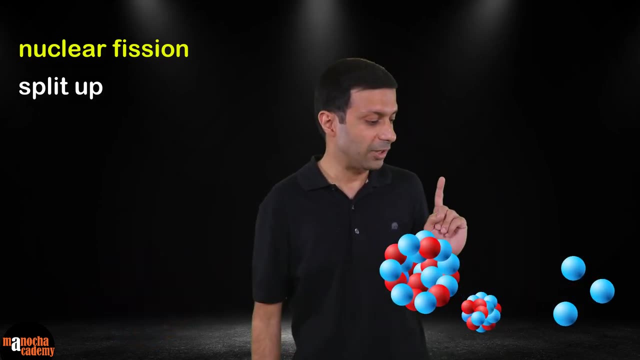 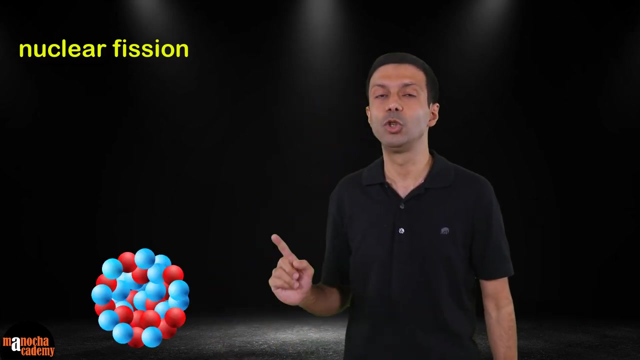 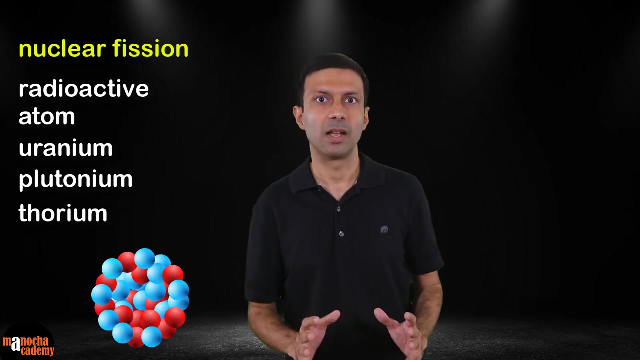 Let's start with nuclear fission. The word fission means to split up, So in nuclear fission a heavy nucleus splits up into two lighter nuclei and it releases a huge amount of energy. The heavy nucleus is usually made of a radioactive atom such as uranium, plutonium or thorium. 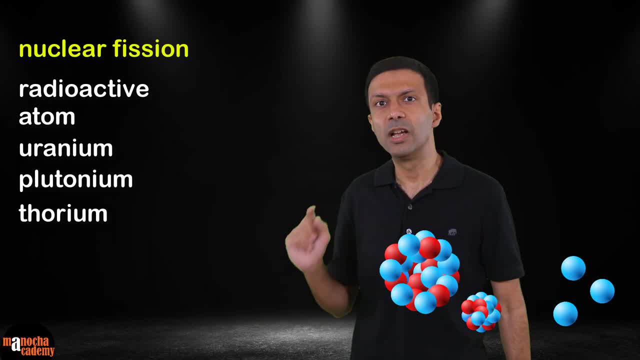 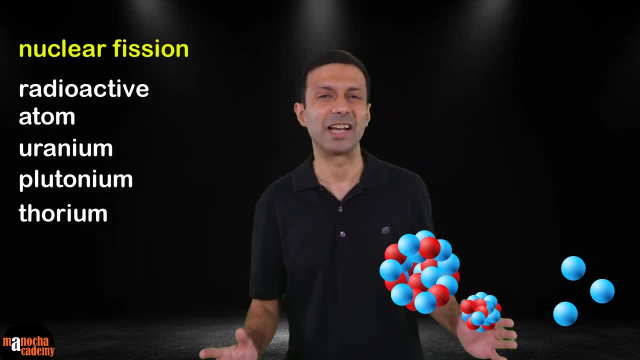 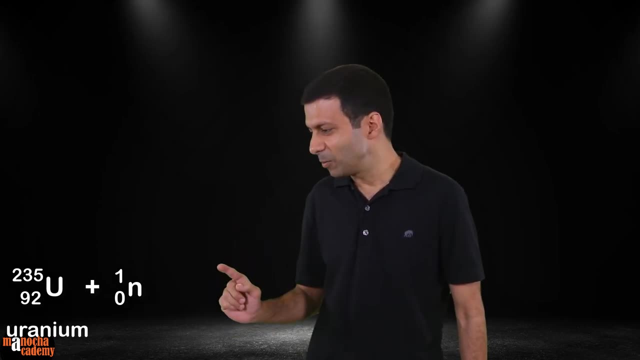 And the heavy nucleus is split up by bombarding it with slow moving neutrons, low energy neutrons. Let's take a look at an example reaction. In this reaction, the heavy nucleus is uranium. Now, when the uranium atom is bombarded with a slow moving neutron, it splits up into two. 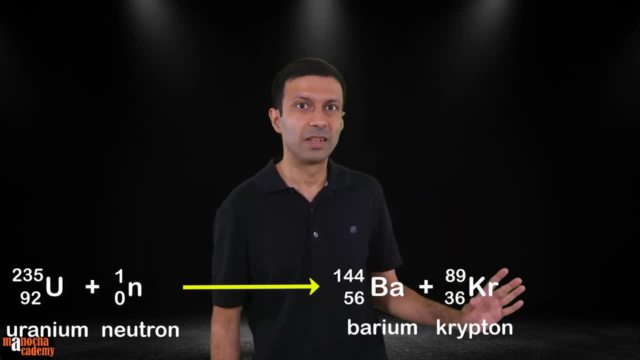 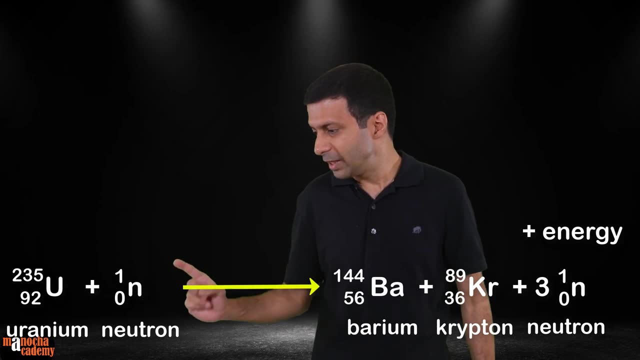 atoms, barium and krypton, Three neutrons are produced and a tremendous amount of energy is released. Now, if you look closely at the fission equation, can you see that there are numbers written next to the symbols of the atoms? Let's look at the fission equation. 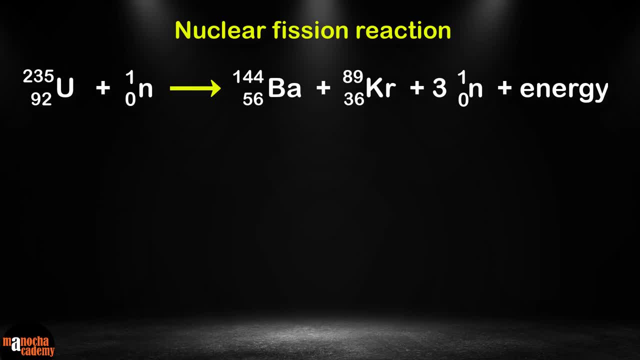 Do you know what these numbers are? That's right. The lower numbers are called atomic numbers and the numbers on top are called mass numbers. Atomic number is the number of protons present in an atom. Mass number is the total number of protons and neutrons present in the atom. 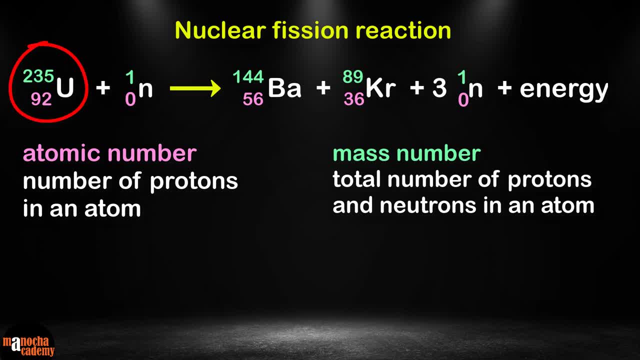 If we take the example of uranium atom in this equation, the atomic number is 92.. So the uranium atom has 92 protons. The mass number is 235.. So uranium has a total of 235 protons and neutrons. Now we can easily work out the number of neutrons in uranium. 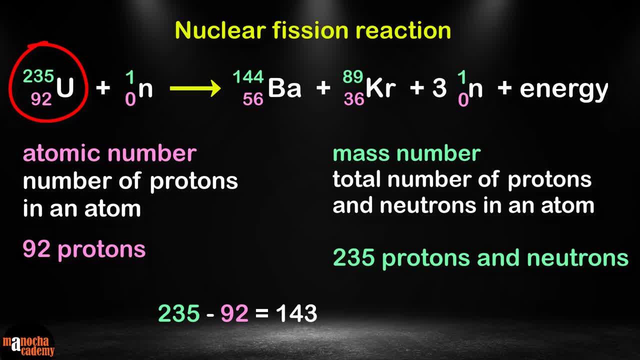 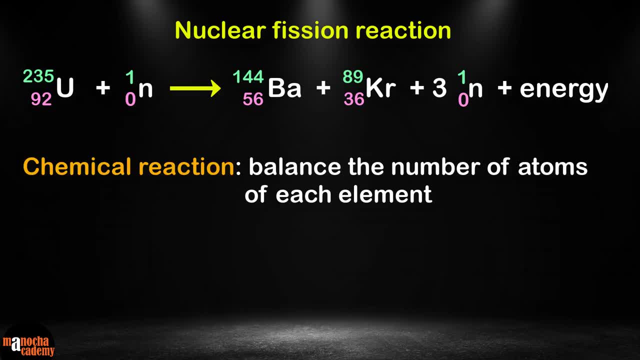 It will be 235 minus 92, which is equal to 143 neutrons. Remember, when we balance a chemical equation, we balance the number of atoms, of each atom. So we can easily work out the number of neutrons in uranium. 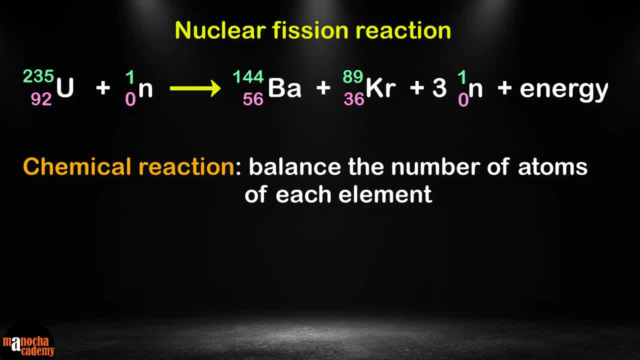 It will be 235 minus 92, which is equal to 143 neutrons. So we can easily work out the number of atoms of each atom. Now, we can't do that in a nuclear reaction because, as you can see, in a nuclear reaction 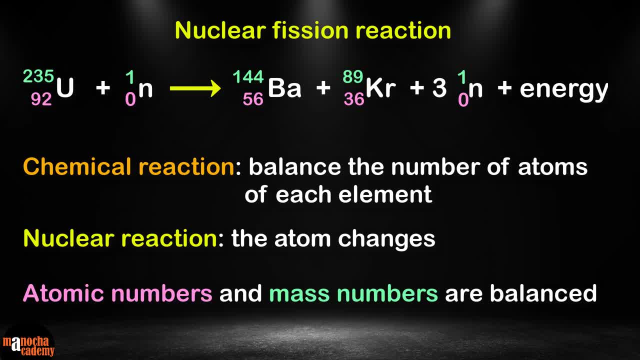 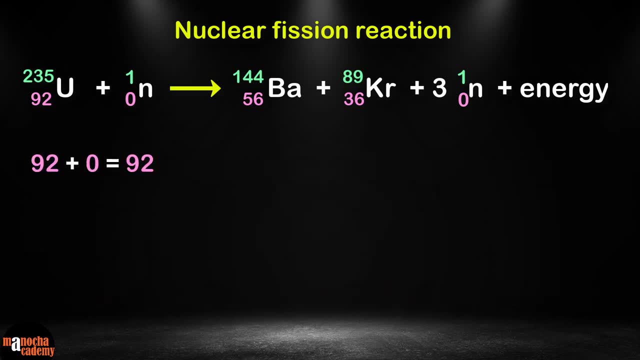 the atom itself changes, But the atomic numbers and mass numbers in the nuclear reaction are balanced. So if you add up the atomic numbers on the left side of this equation, as you can see, it will be 92 plus 0, which is 92.. 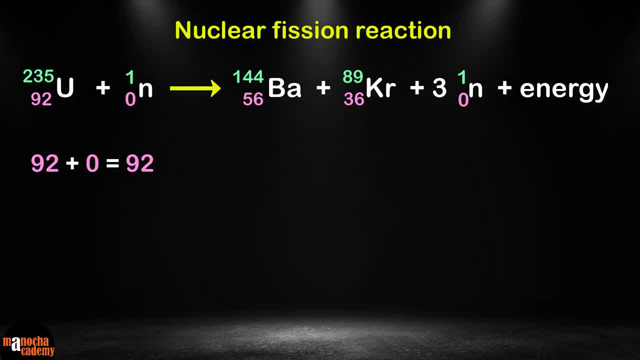 And the sum of the atomic numbers on the right side of this equation will be 92 plus 0, which is 92.. And the sum of the atomic numbers on the right side is equal to 56 plus 36 plus 3 into 0,. 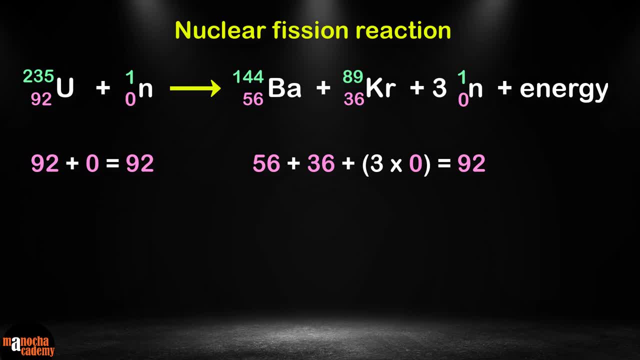 which is 92. So the atomic numbers on the left and right side are equal. Similarly, if you add the mass numbers on the left side, the sum is 235 plus 1, which is equal to 236.. And the sum of the mass numbers on the right side is equal to 144 plus 89 plus 3 into 1,. 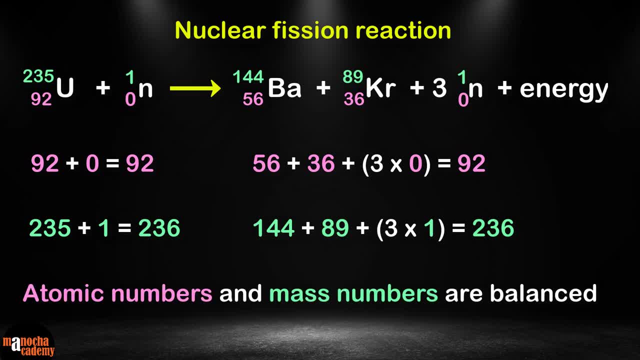 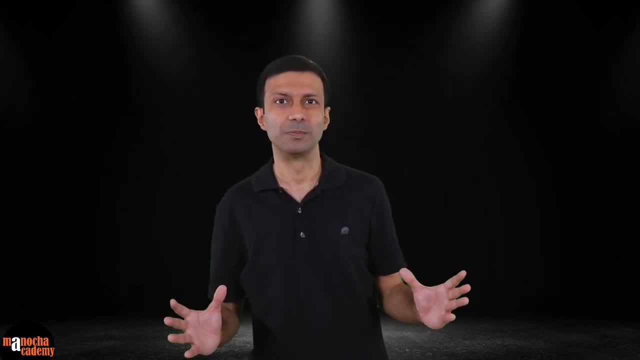 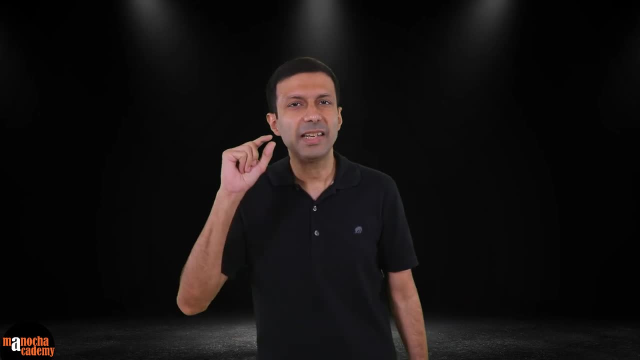 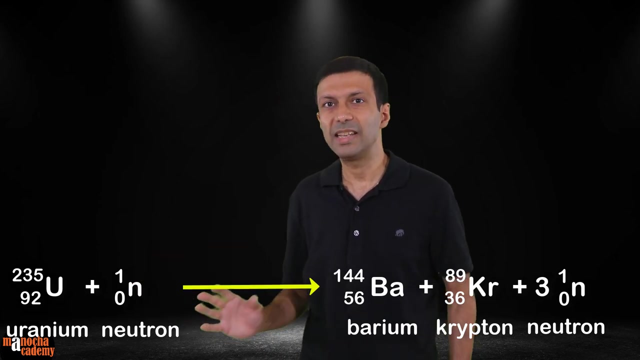 which is also 236.. So the mass numbers are also balanced. Then where does the energy come from? Even though the atomic and mass numbers of a nuclear reaction are balanced, there is still a tiny loss in mass. The total mass of the reactants, which is uranium and the neutron, is slightly more. 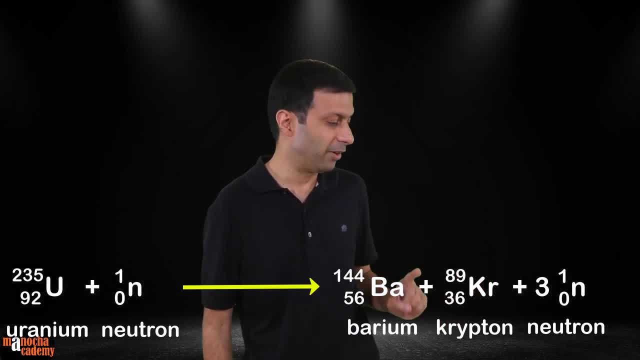 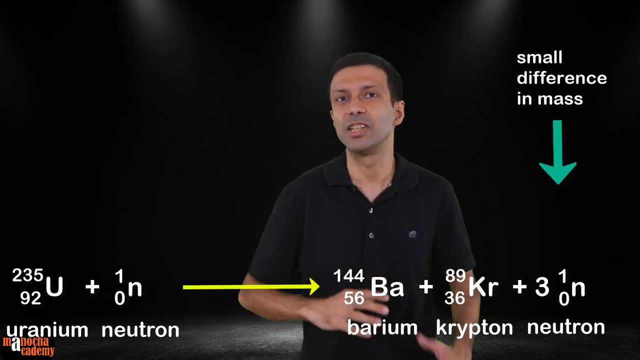 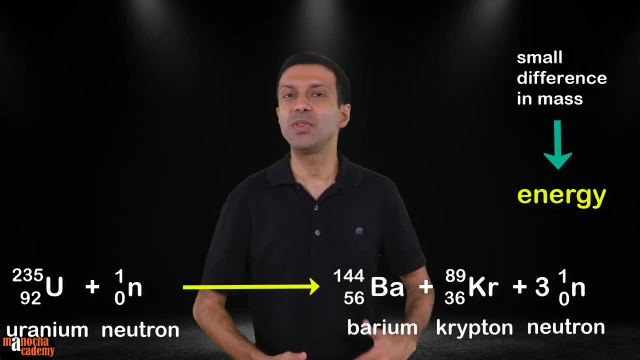 than the total mass of the products here, Which is barium, Crypton and these three neutrons. Now this small difference in mass is converted to energy, And this is the nuclear energy obtained from nuclear fission. As we discussed, we can calculate the amount of energy using Einstein's famous formula. 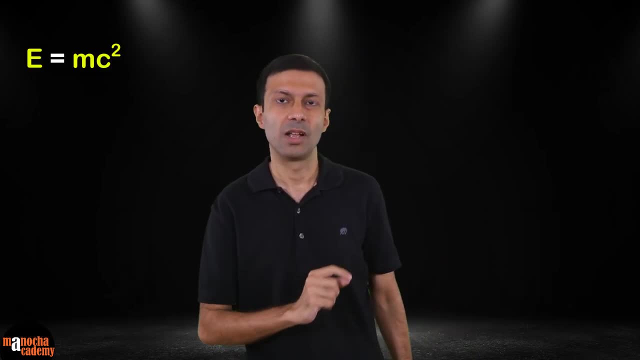 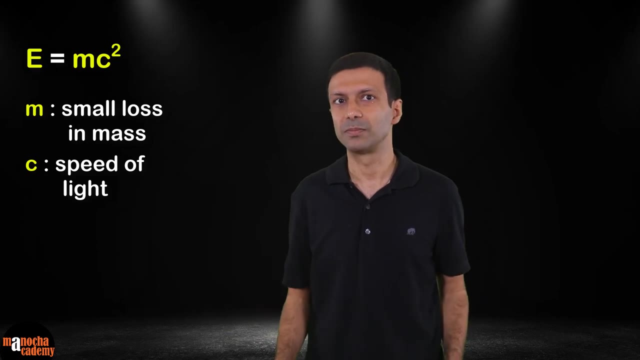 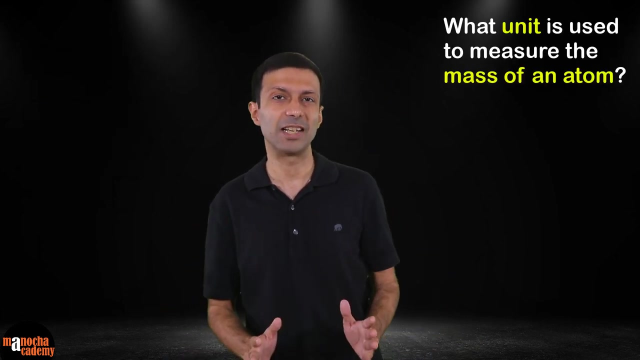 E equal to mc square, where m is the small loss in mass in the reaction and c is the speed of light. Now the SI unit of mass is kg. But what is the convenient unit that is used to measure the mass of an atom? 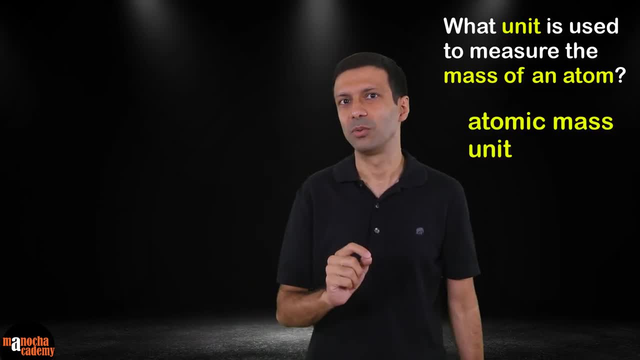 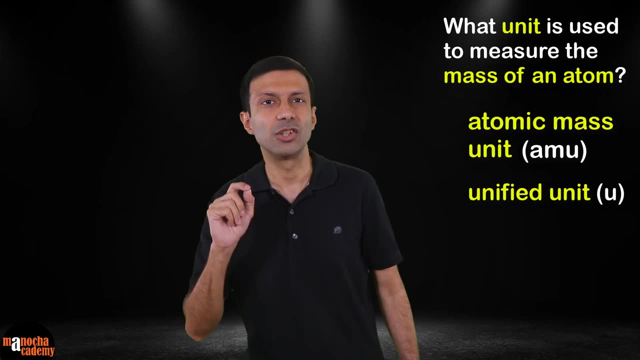 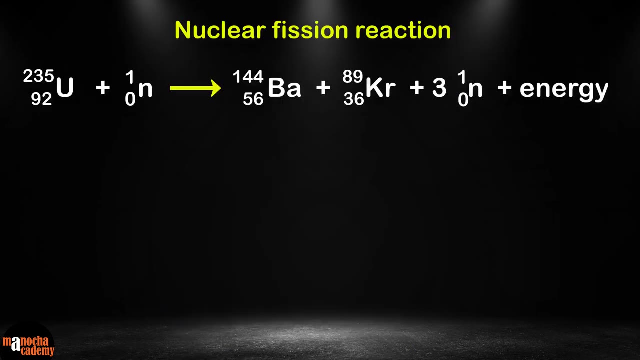 That's right. it's called the atomic mass unit, which is written as amu, And it's also known as the unified unit, which is written as u. Now let's look at the loss in mass in amu in this fission reaction. 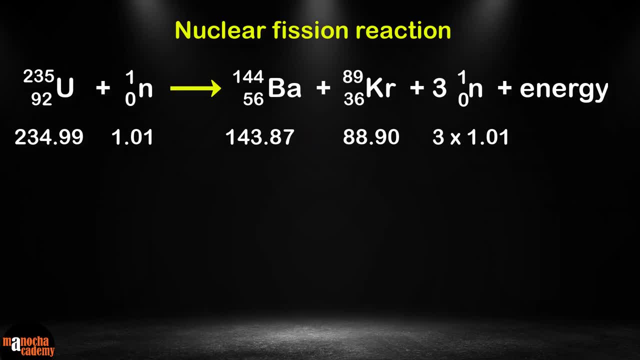 Here is the mass of each atom in amu And the mass of a neutron. Here is the mass of each atom in amu And here is the mass of a neutron. So the loss in mass in this fission reaction equals the mass of the uranium nucleus plus. 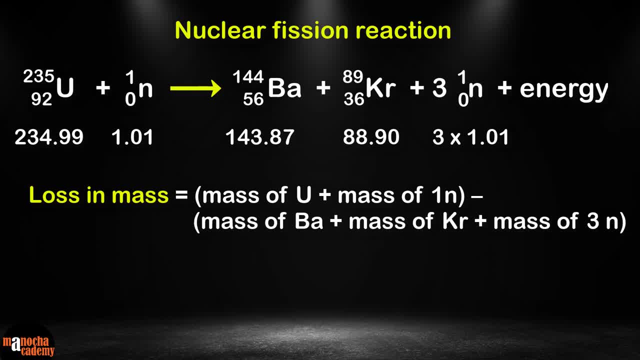 mass of one neutron minus mass of the barium nucleus plus mass of crypton nucleus plus mass of three neutrons. Now if we plug in the numbers, we get the loss in mass for this reaction as 0.2 amu or 0.2 u. 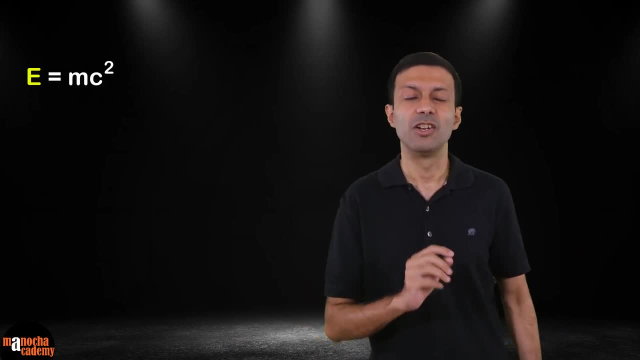 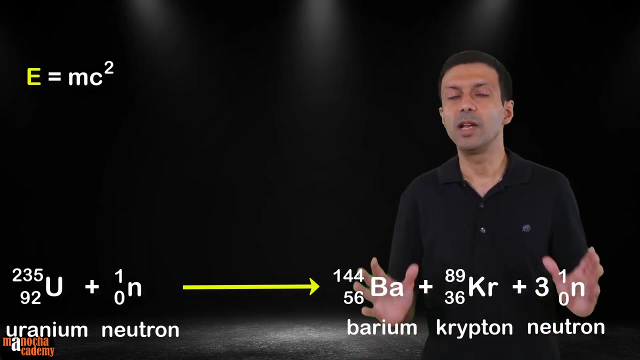 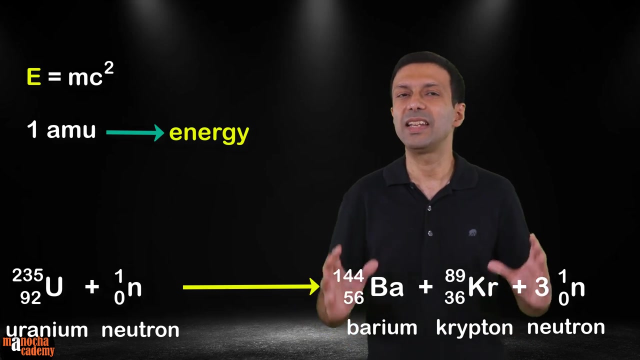 We can use Einstein's equation E equal to mc squared to calculate the amount of energy released in this nuclear reaction. Now it'll be convenient to know the amount of energy released when one amu of mass is converted into energy. Then we can easily calculate the energy for this reaction or for any other nuclear reaction. 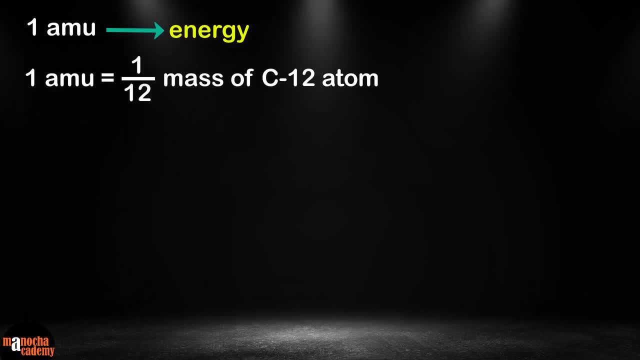 We know that one amu is equal to one twelfth the mass of a carbon-12 atom. So this is equal to 1.66 into 10, to the power minus 27 kg. Now let's use Einstein's equation E equal to mc squared to calculate the amount of energy. 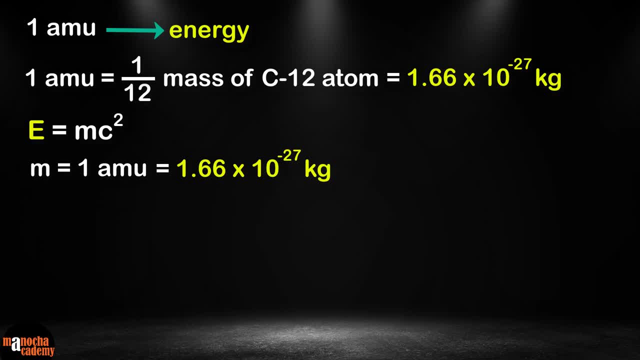 Let's substitute the loss in mass m and speed of light equal to 3 into 10 to the power, 8 meter per second. Note, it is the square of the speed of light here, And multiplying the numbers we get Energy equals 1.49 into 10 to the power, minus 10 joule. 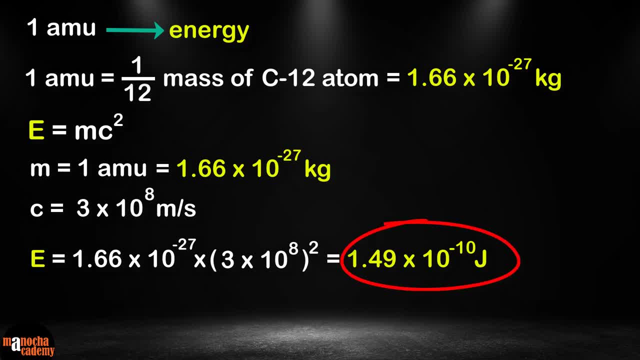 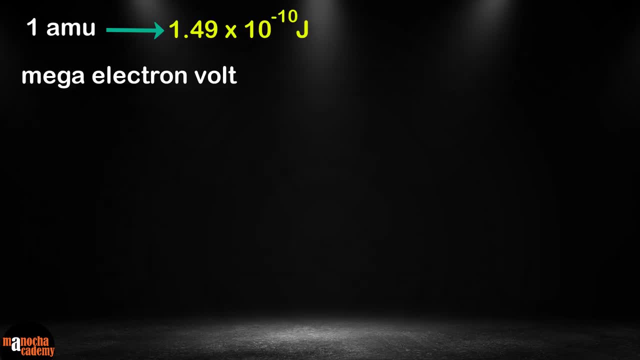 So loss in mass of one amu gives us this much of energy in joules. Usually a more convenient unit called mega electron volt, or MeV in short, is used for nuclear energy. One mega electron volt equals 1.6 into 10 to the power minus 13 joule. 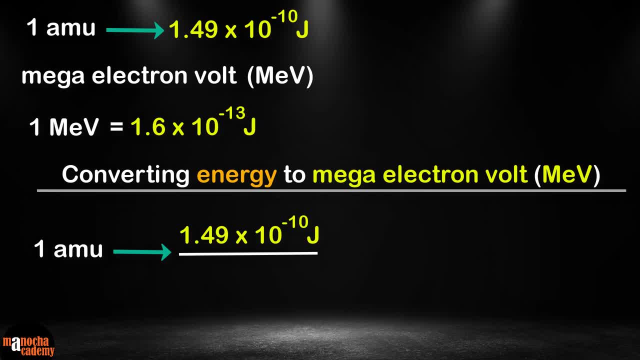 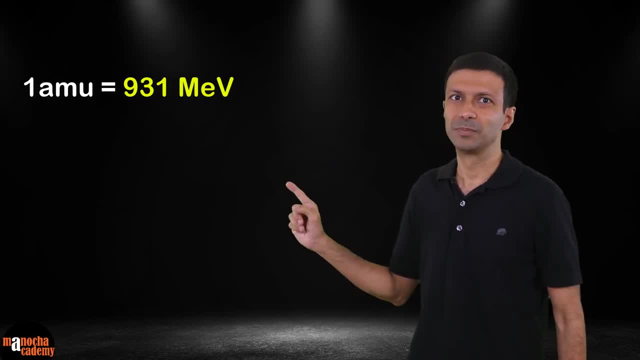 So if we convert this Energy in terms of mega electron volts, we are going to get 931 MeV. This is a really useful number to remember. If in a nuclear reaction there is a loss in mass of 1 amu or 1 u, then the amount of energy 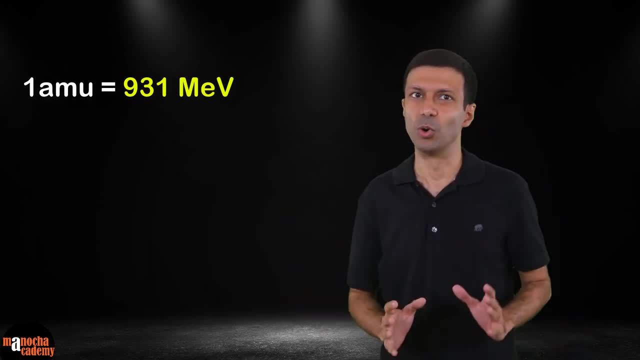 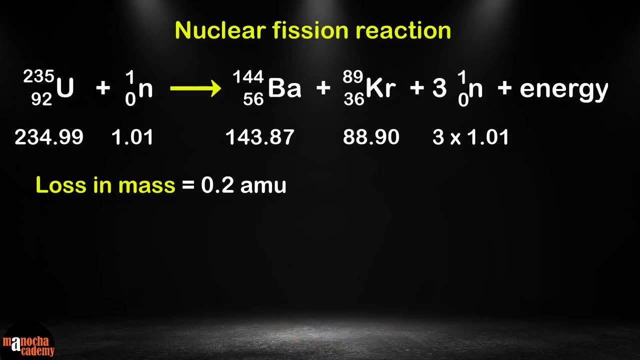 released is 931 mega electron volt. Now we can easily calculate the amount of energy for our fission reaction. It will be 0.2 into 931 mega electron volt. 0.2 into 931 mega electron volt. 0.2 into 931 mega electron volt. 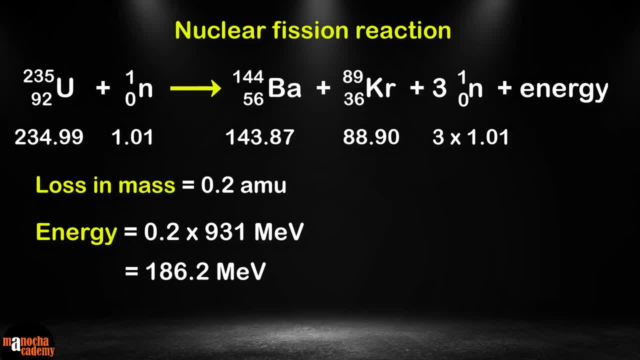 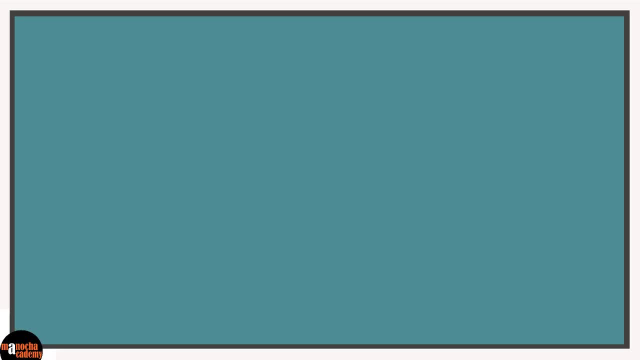 So this student here. he took the meu of energy. this amount is the one mu of energy in square of the electricity obtained from he 그다음. So now we have alone 186.2 MeV of energy. Let's place Einstein's mass energy equation and these important numbers: 1 amu, equal to 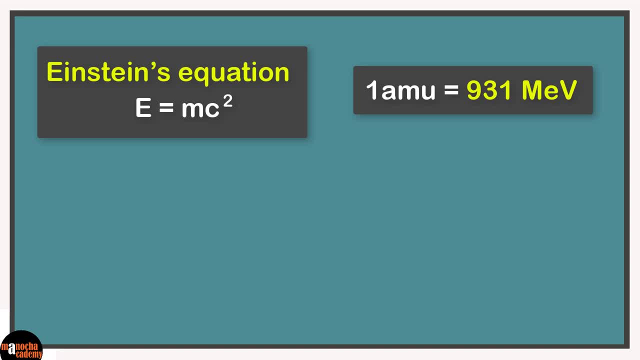 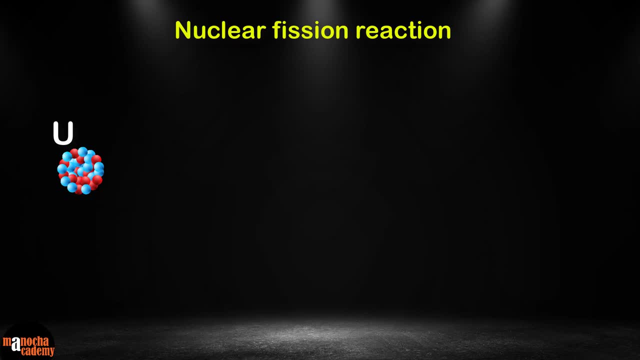 931 mega electron volt on our concept board. An interesting thing about the nuclear fission reaction of uranium 235 is that one neutron is used to fission, used to cause the fission, and three neutrons are produced by the fission. Now, these three neutrons: 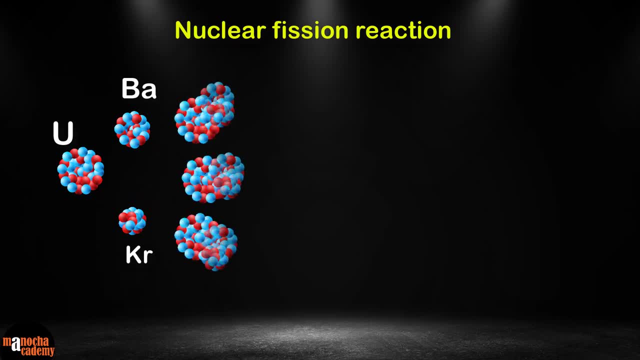 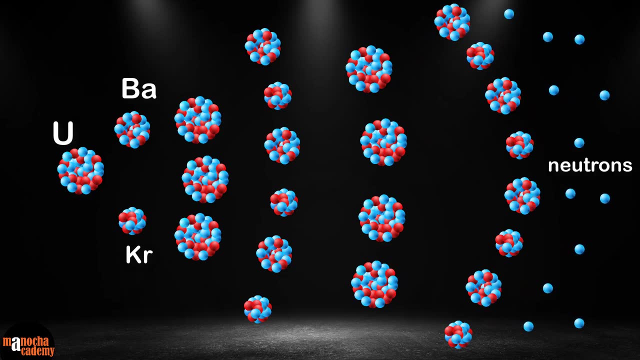 which are produced can split three more uranium atoms and again, for each uranium atom, three more neutrons will be produced, as shown here. Now, this is a self-sustaining reaction because it can go on and it's called a chain reaction. Now, if this chain reaction is allowed to go on in an 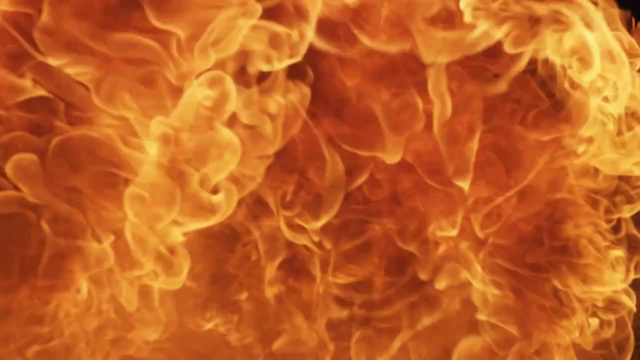 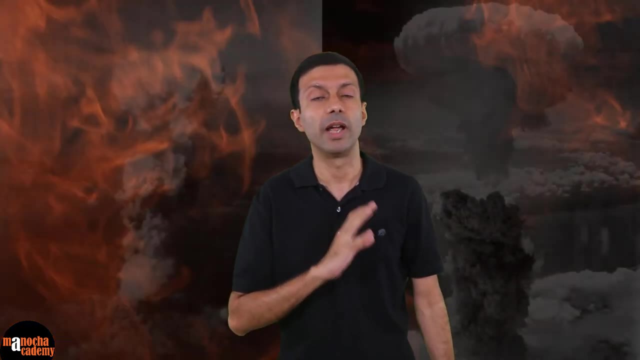 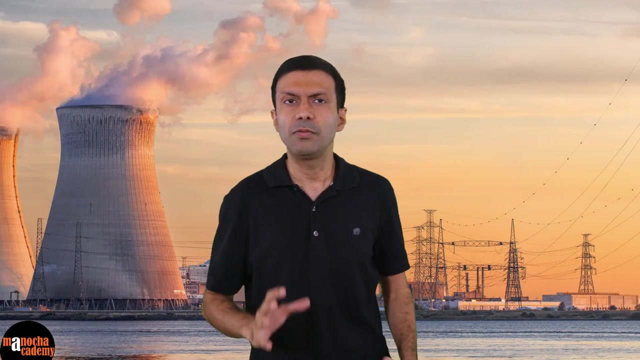 uncontrollable way, then it's an atom bomb. It produces a massive amount of energy. The atom bombs that were dropped on Hiroshima and Nagasaki during the second world war were nuclear fission bombs. But if the chain reaction is controlled in some way, then it can be put to. 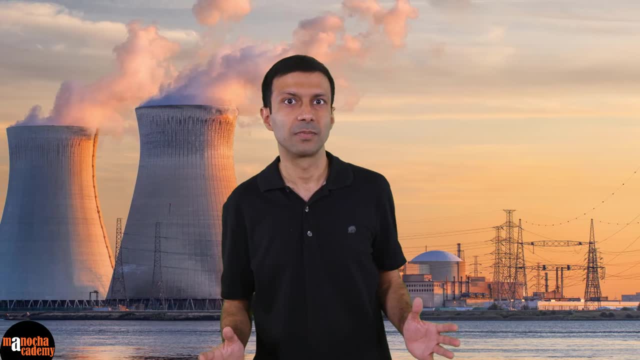 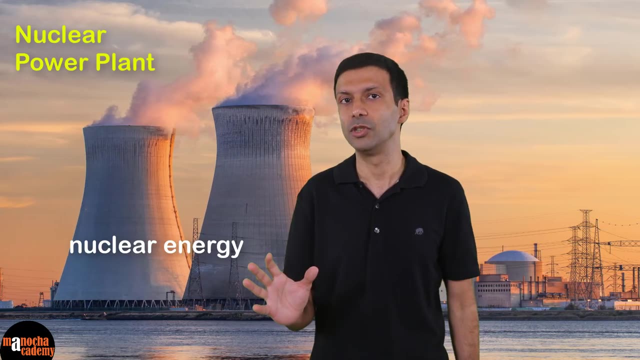 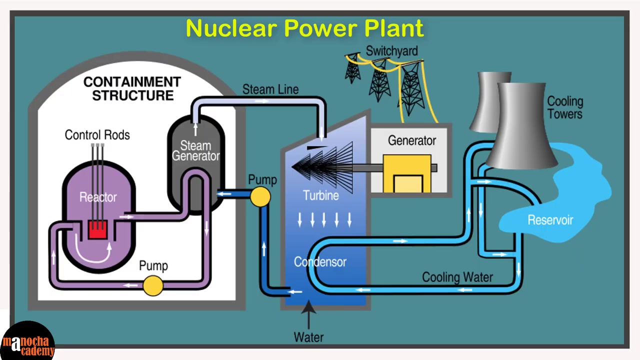 good use and generate electricity, And this is done in a nuclear power plant. The goal of the nuclear power plant is to use nuclear energy to produce electrical energy. A nuclear power plant looks something like this, As you can see, on the left side there's the nuclear reactor. This is where the nuclear fission. 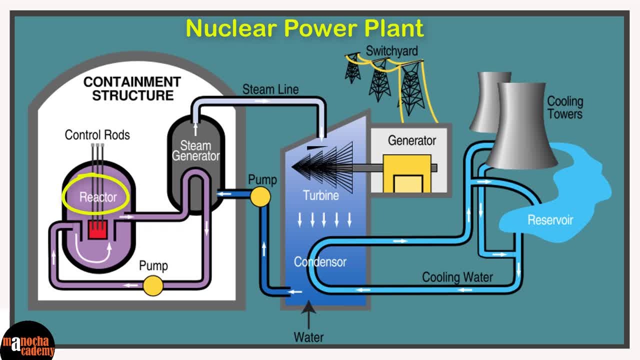 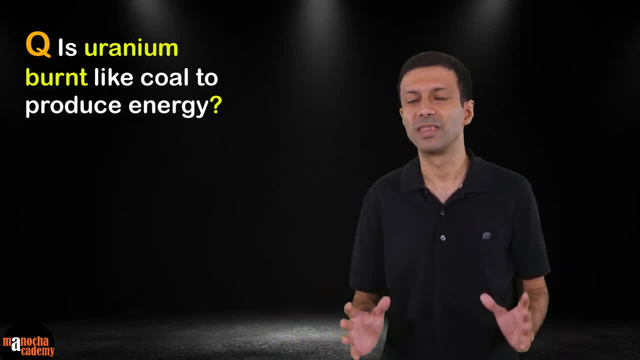 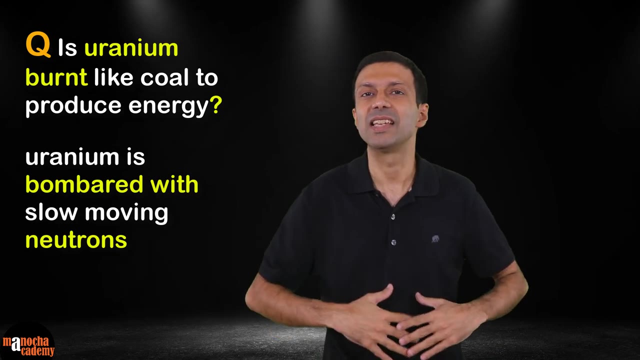 Is the uranium fuel burnt like coal to produce energy? That's right. Uranium is not burnt, As we discussed. to achieve nuclear fission, uranium is bombarded with slow moving neutrons so that it splits up and releases energy. The fission of uranium is carried out in a steel pressure vessel. 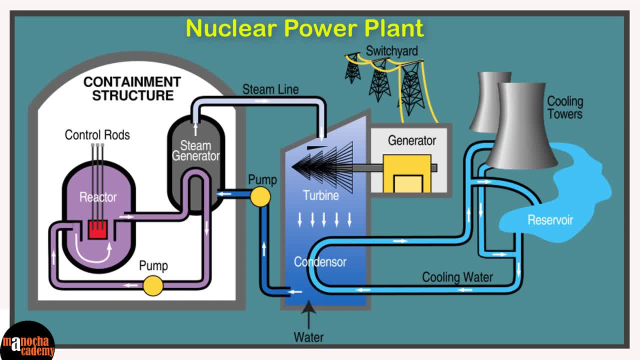 Now the uranium rods are inserted in a core made of graphite. Now what we're looking at are graphite blocks, which is inside the reactor. Now, graphite is a moderator. Graphite slows down the speed of neutrons, since slow moving neutrons are needed for fission, And boron rods are placed between the uranium rods. The Boron rods are 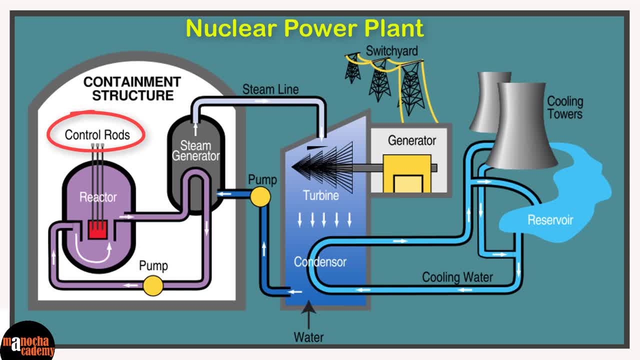 called control rods Because they absorb excess neutrons and control the chain reaction. Now, if there are no control rods, then they're just économics rods, anddollar- These are programmes of governmentite rods. then the chain reaction will go out of control and it can lead to an explosion. 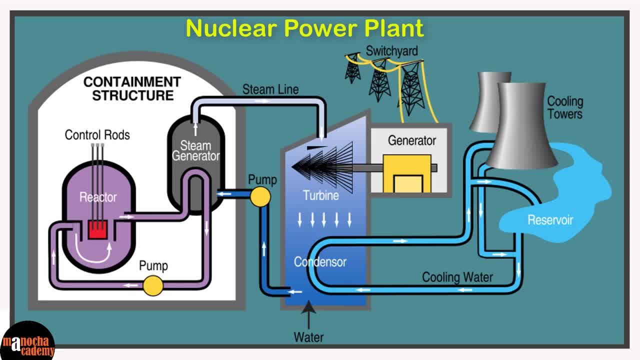 Since nuclear fission also produces harmful radiations, the reactor is enclosed in a concrete chamber made of thick walls to absorb these harmful radiations. Liquid sodium or carbon dioxide gas is used as a coolant to transfer the heat produced in the reactor to the heat exchanger. 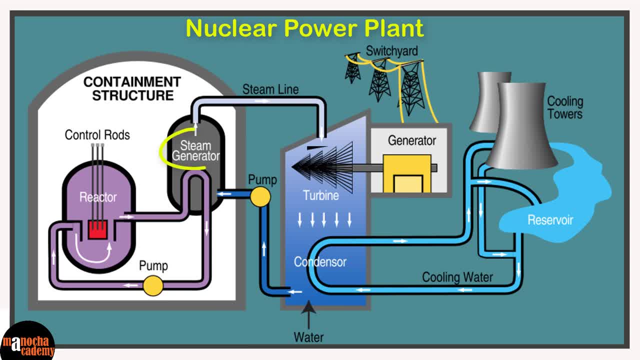 The water absorbs the heat and boils into steam. The hot steam at high pressure is used to turn the turbine, And the turbine rotates and drives the generator, which produces electricity for us, And the used steam is condensed back into water and it is recycled back. 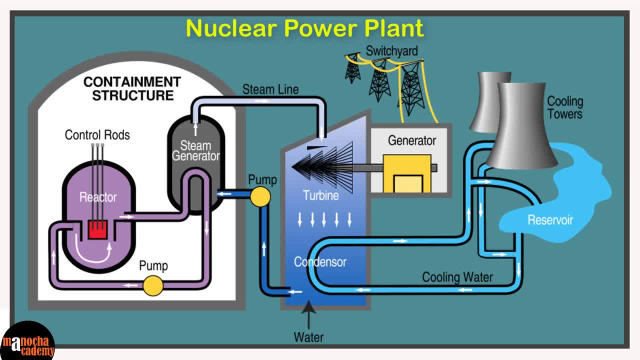 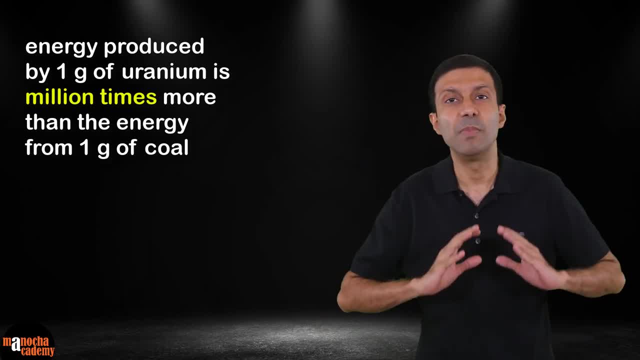 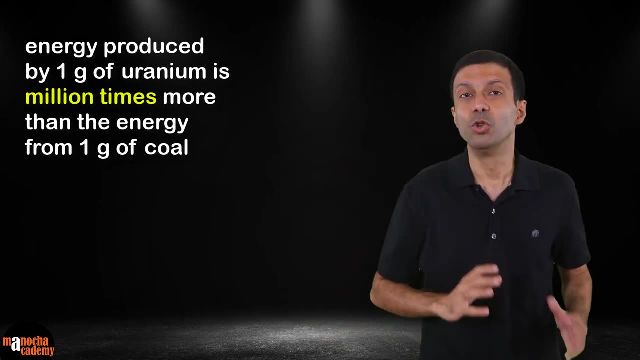 So this is how our nuclear power plant works. Did you know that the energy produced by 1 gram of uranium from nuclear fission is million times more than the amount of energy produced by burning 1 gram of coal? So nuclear power plants are very efficient and can produce a lot of energy. 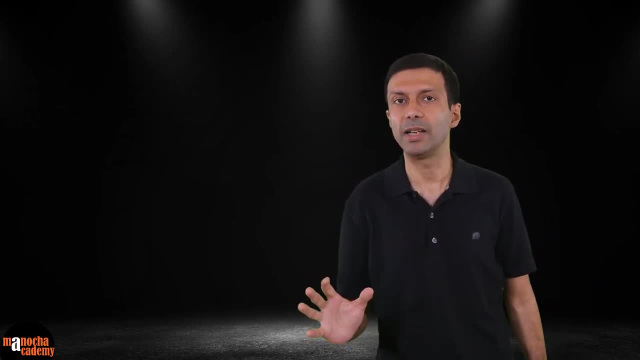 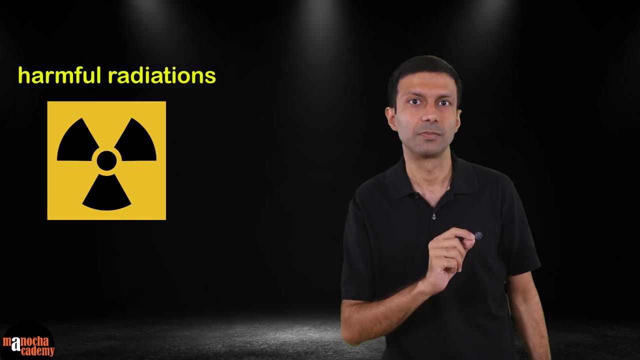 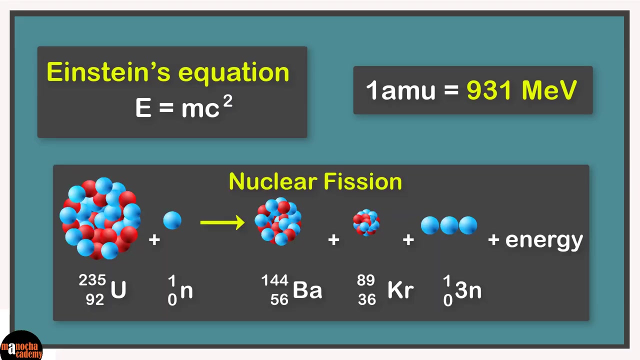 However, the products of nuclear fission that are left behind are extremely harmful, since they are radioactive and they produce harmful radiations. These products are called nuclear wastes And a lot of care and precaution has to be taken to dispose the nuclear waste materials. Lets go ahead and place nuclear fission on our concept board. 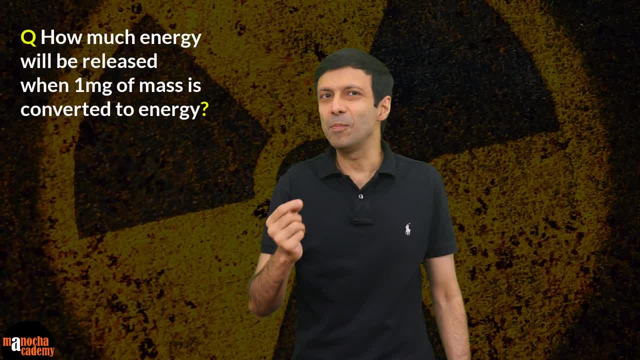 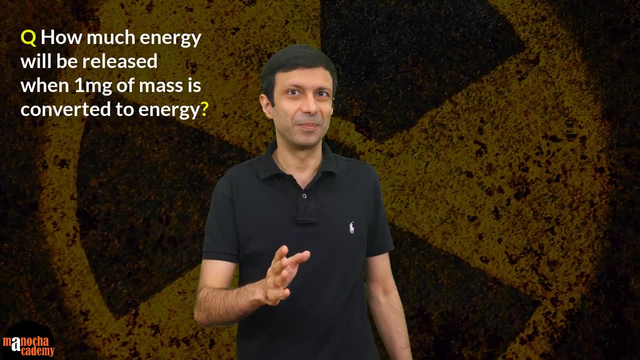 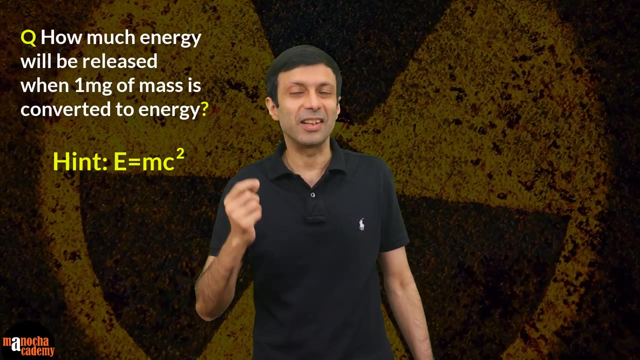 Now I have a quiz question for you. Suppose 1 milligram of mass is converted into energy. Can you calculate how much energy will be released? Remember, We need to use Einstein's famous equation E equal to mc2 to calculate the amount of. 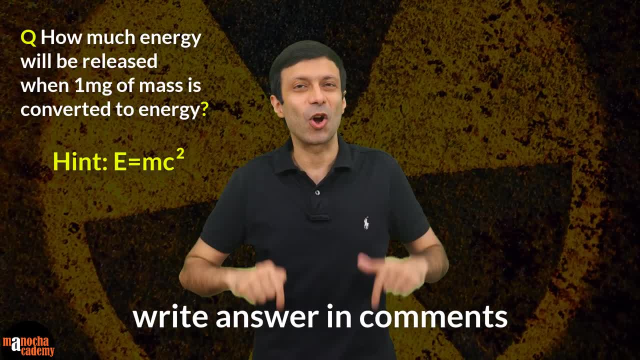 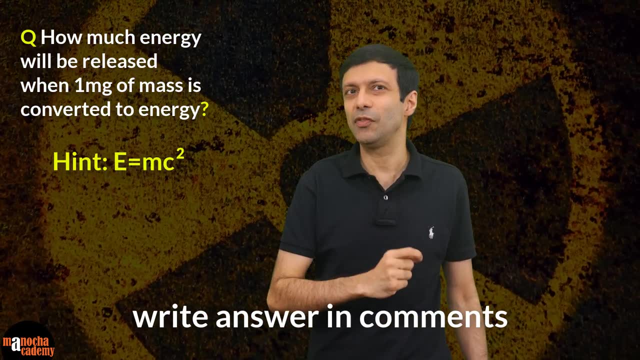 energy. So do let me know your answers by putting it in the comments below, And I promise to reply to your answers. So go ahead and try this question that: how much energy will be released if 1 milligram of mass is converted into energy?